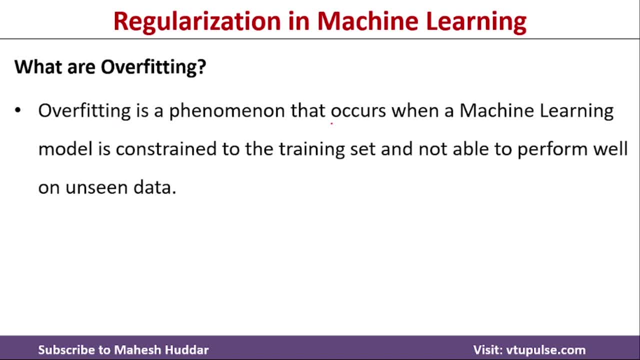 is Overfitting here. Overfitting is a phenomena that occurs when machine learning model is constrained to the training set. That is nothing, but the model is working fine on the training set, but not on the testing or the validation data. It is also known as unseen data here. 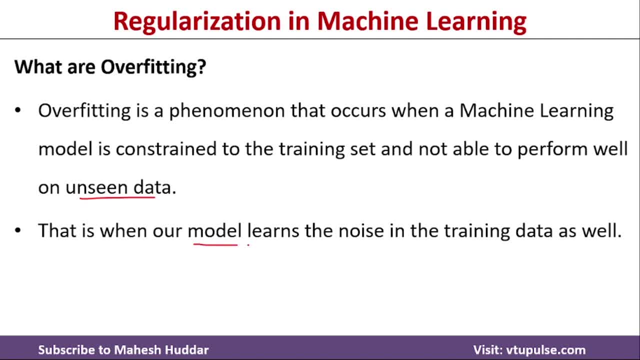 This kind of situation occurs in machine learning, because the model learns the noise in the training data as well as the model memorizes the training data instead of learning the data. This is the reason why the model is not working properly on the training data. The same thing it tries to replicate on the testing data, because the testing data is unseen. 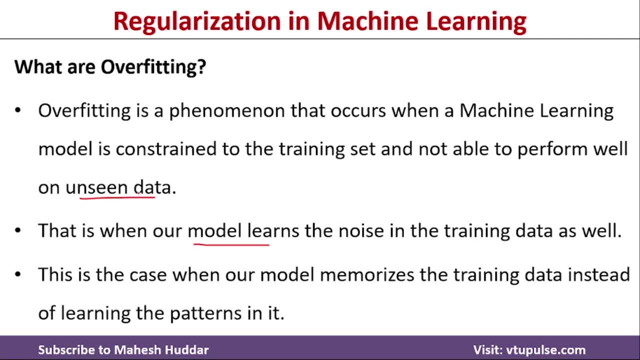 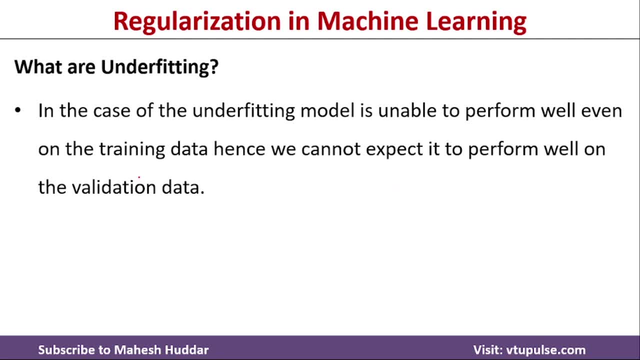 data. It may not work properly on the testing data. over here Now we will define what is underfitting. Underfitting model is unable to perform well on the training data. also, The meaning of this one is the model which doesn't works well on the training. 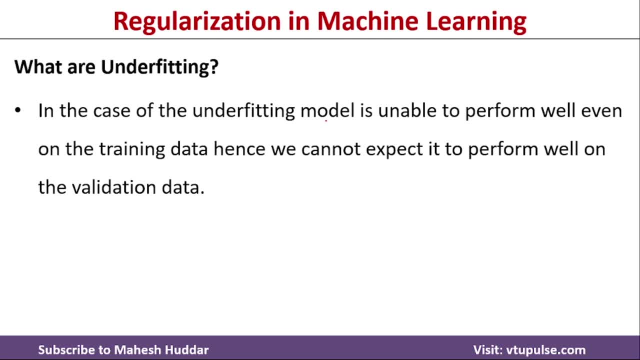 data. that is called as the underfitting model. If it is not working well on the training data, we cannot expect it to perform well on the validation or the testing data here. In this case, we need to increase the complexity of the model or we need to add more features to the feature set so that 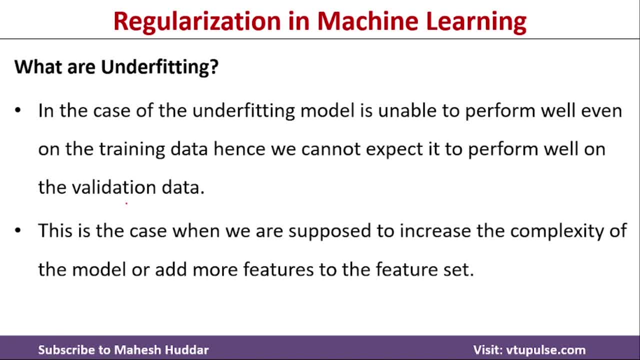 the model performs well on the training data. If it starts working well on the training data, then we concentrate on the other side, that is, whether it works fine or not on the validation or the testing data over here. These are some of the examples for the underfitting, overfitting and 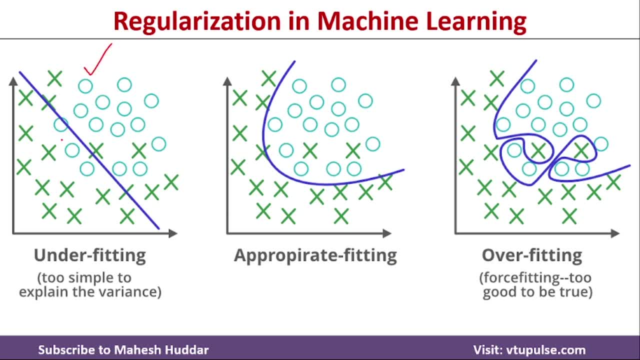 appropriate fitting here. If you look at this particular first one, this particular model is performing very poor on the training data. Because of that it is called as underfitting. It is too simplistic model. Many of the examples were classified or can say that incorrectly classified over. 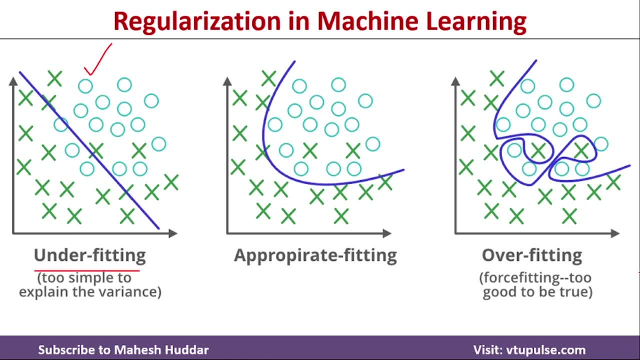 here. So that's the reason it is called as the underfitting here. When you consider this particular model, this particular model has learned too much. in this case It has very. you can say that the sharp edges, or you can say that the high sharp edges. It can say that the sharp edges, or it can say that the 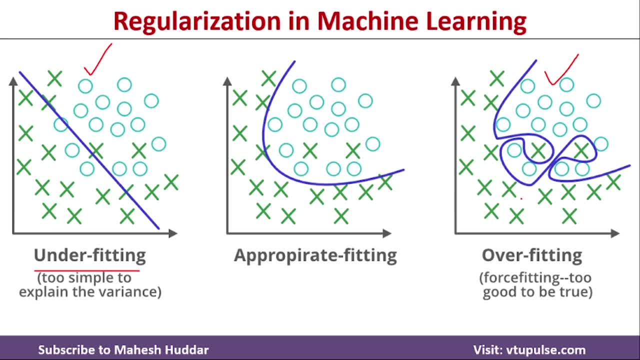 hyper plane. Because of that, you can say that it is a overfitting situation. It is trying to memorize the training data rather than learning from this particular training data over here. When it comes to this particular example, in this case, the model has learned a bit. There are few misclassifications, are there? 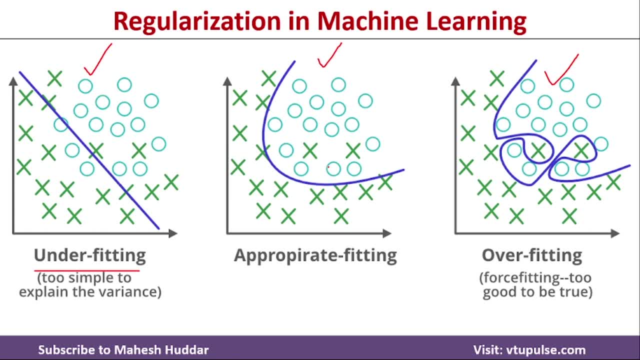 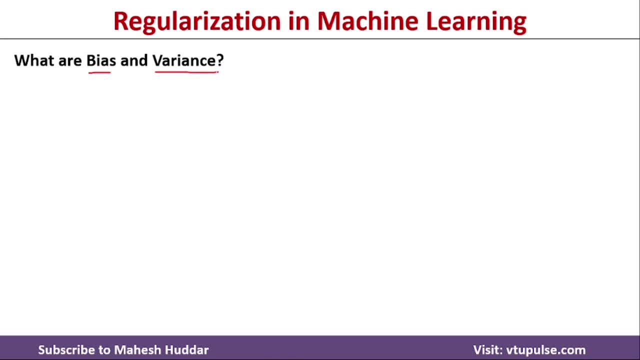 but it is, you can say that, the appropriate fitting for the given training data over here. Now we will define two more very important terms. One is called as bias, The other one is called as variance. here Bias refers to the errors when we try to fit a statistical model on the real world data which does not fit perfectly well on some of the mathematical models here. 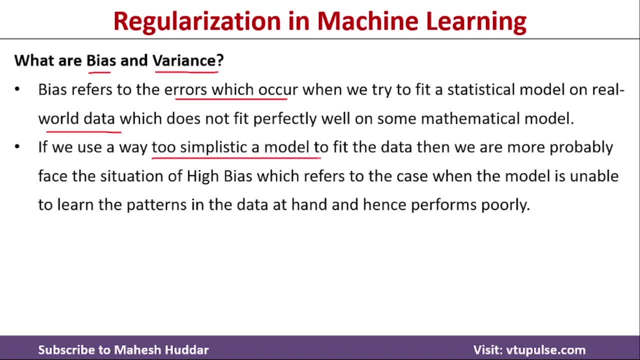 Let us say that we have chosen a very simplistic model to fit the given training data. Many times what happens is the model is unable to learn from the patterns in the given data, hence perform poorly on that particular data. Such a situation is known as the high bias here. That is nothing. but whenever we have chosen a very simplistic model, it may not perform well on, we can say that the training data- Such a situation is known as the high bias over here. 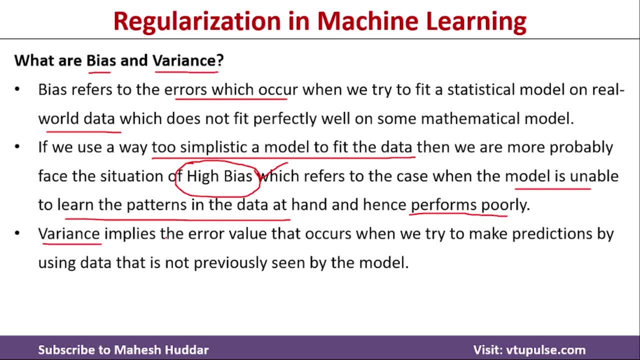 The second one is variance. Variance implies that the error value that occurs when we try to make predictions by using data that is not previously seen by the model, That is nothing, but the variance implies that the error value that occurs when we try to make predictions by using data that is not previously seen by the model. 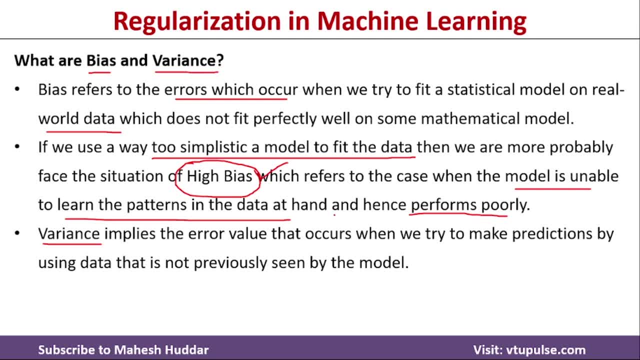 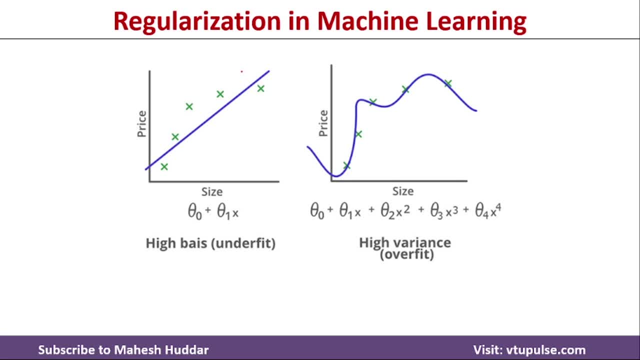 In the first case we have chosen a very simplistic model that is nothing but the linear regression In this particular case. so many of the examples we have not fitted properly here, so definitely we will get maximum error on the training data. Such a situation is called as underfitting, as well as high bias over here. When it comes to second one, the model is trying to learn too much from the training data. Because of that, such a situation is known as overfitting here. It's also known as high variance over here. 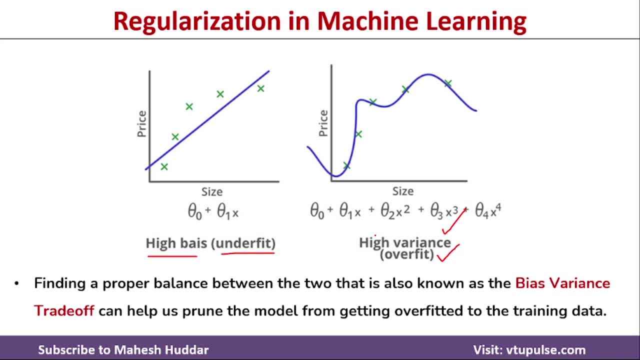 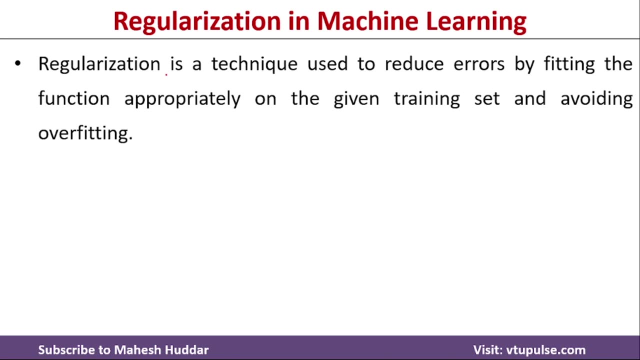 Finding a proper balance between these two, that is, high bias and high variance is also known as bias variance trade-off. that is the very important part of machine learning model. here Now we will discuss what is actually regularization in machine learning and what are the different techniques to. 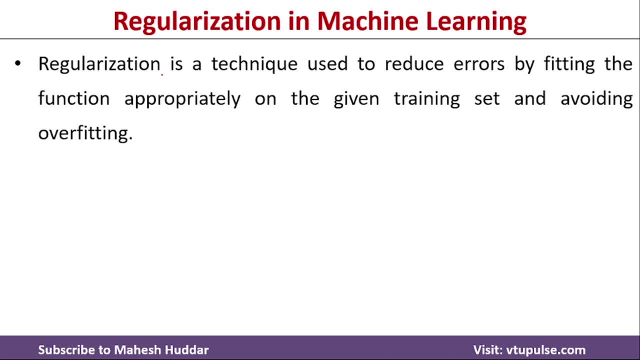 achieve regularization in machine learning. Regularization is a technique used to reduce the errors by fitting the function appropriately on the training set and avoiding the overfitting over here. So what we do here is we will try to fit our model on the training set appropriately. 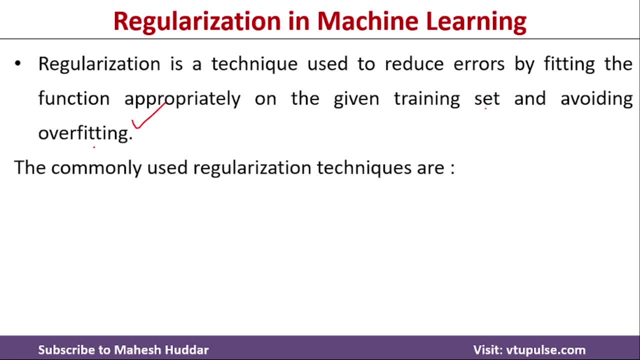 in such a way that we avoid overfitting. in this particular case, There are mainly three regularization techniques are available. One is known as lasso regularization, also known as L1 regularization. Second one is known as ridge regularization, also known as L2 regularization. 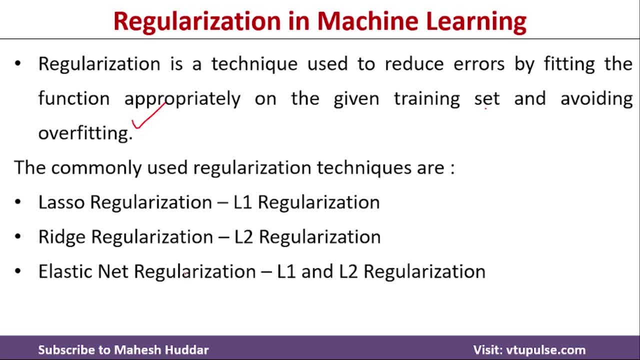 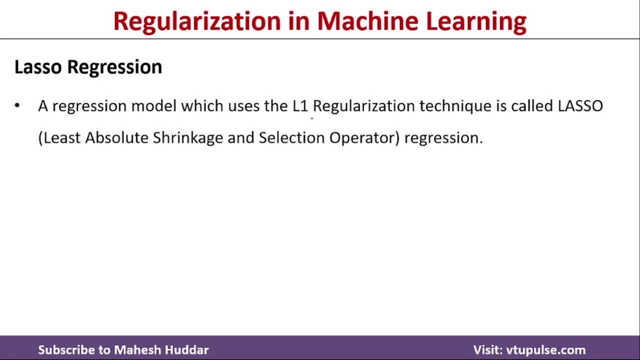 Third one is known as elastic net regularization, also known as L1 and L2 regularization in this case. First we will try to understand the lasso regularization here. Lasso regression is a regression model which uses L1 regularization technique, which is known as least absolute. 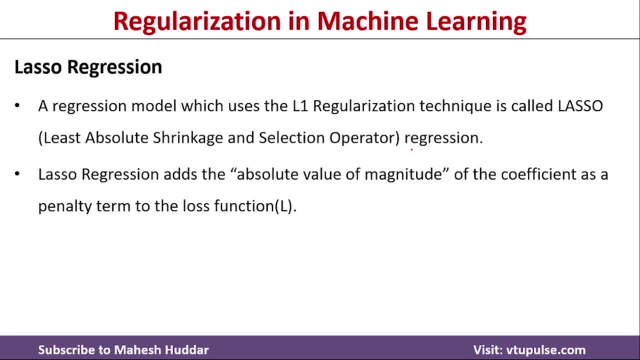 shrinkage and selection operator regression. In this case we add absolute value of magnitude as a coefficient of a penalty term to the loss function. Whenever we build any regression model, we will get the error term. That error term is also known as the loss function in. 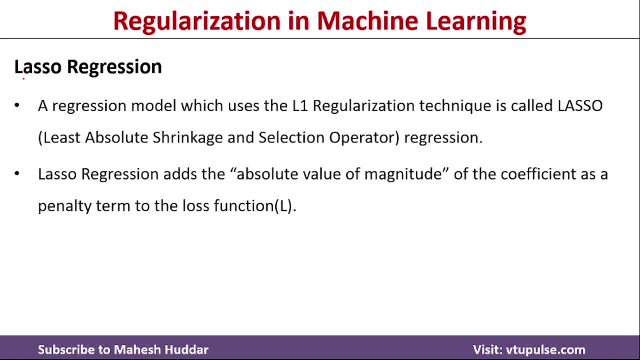 regression terms. So what we do in this lasso regression is we add absolute value of magnitude as the penalty to this particular loss function so that we can reduce that particular loss on the training side as well, as we can say that on the testing side over here. 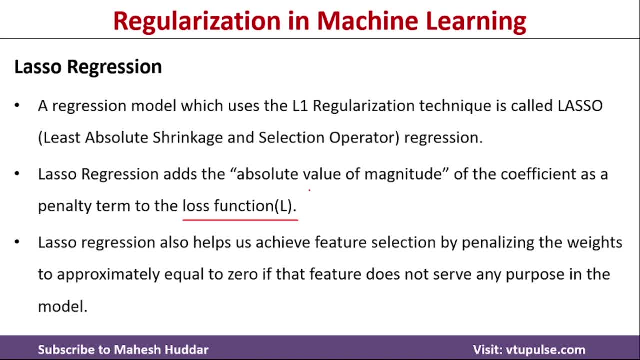 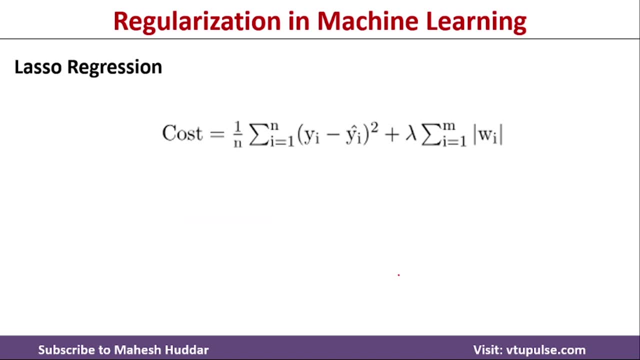 This particular lasso regression helps us to achieve the feature selection by penalizing the weights to approximately equal to 0 if that particular feature is not at all important for that particular model. The lasso regression's loss function looks something like this: This first term: 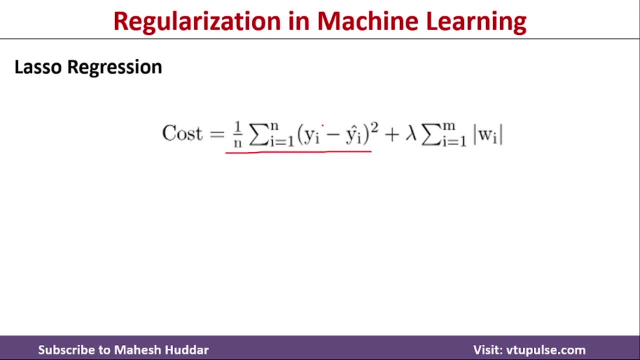 is actually the loss function of a regression model. To this particular loss function we are adding absolute value here. So in this particular case is the number of features here? n is the number of examples given to us. y- i is the actual, or you can say that the target value y i cap, or you can say that y i hat is the predicted target value in this. 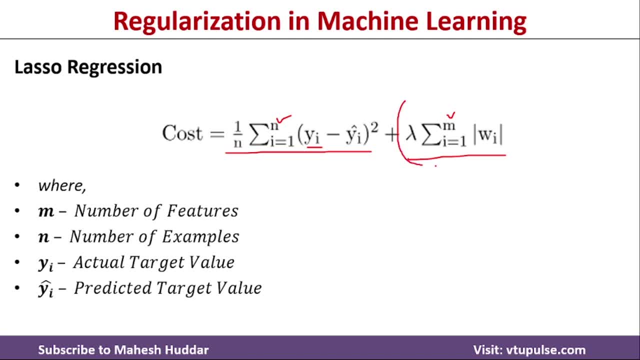 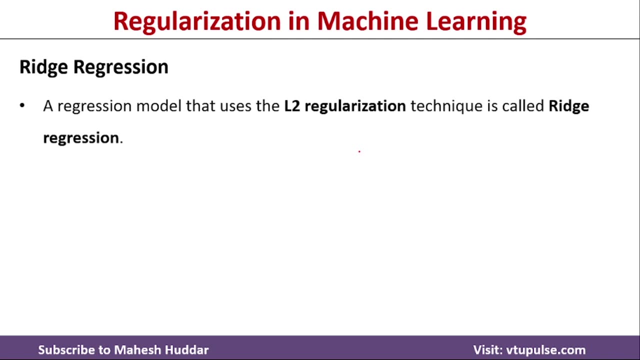 particular case, to this particular loss value, we are adding this particular- we can say that- the penalty term, so that we can reduce the error over here. the second one is known as ridge regression. ridge regression uses something called as l2 regularization technique. ridge regression adds squared magnitude, rather than adding absolute magnitude, to the coefficient function as a. 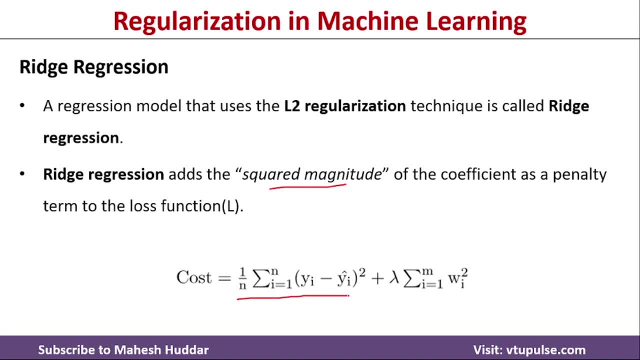 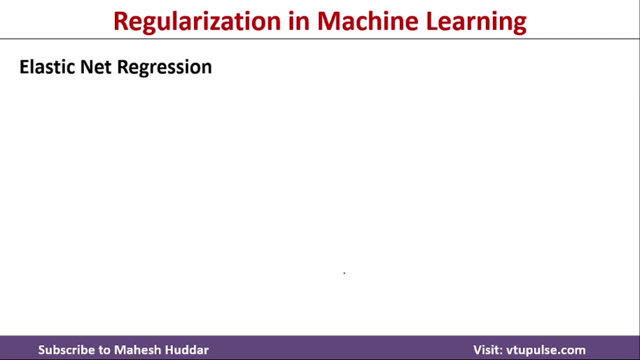 penalty here. so it looks something like this: this is the original loss function. to this particular thing we are adding the squared magnitude over here. coming back to the last one, that is, elastic net regression, elastic net regression is the combination of both l1 as well as l2 regularization. 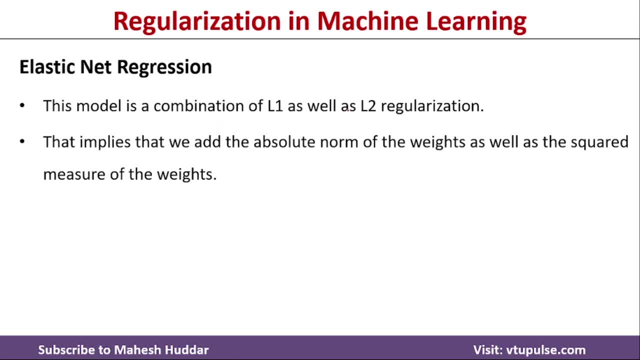 we add these two, l1 and l2, proportionately with the help of another hyper parameter. you can say that alpha over here. the cost function looks something like this: this is the original cost function to this particular thing we are adding. the first one is- you can say that, absolute weight. 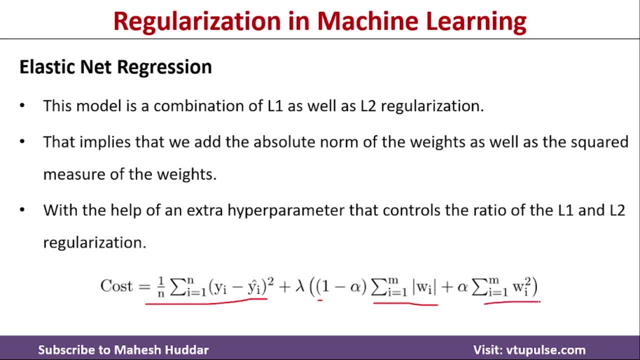 here, and this is the squared magnitude, or the weight here. and we have added one more hyper parameter, in this case, that is one minus alpha, and here we have added alpha here, so alpha can be any value in the range of 0 to 1. if alpha is equivalent to 0, we have something called as 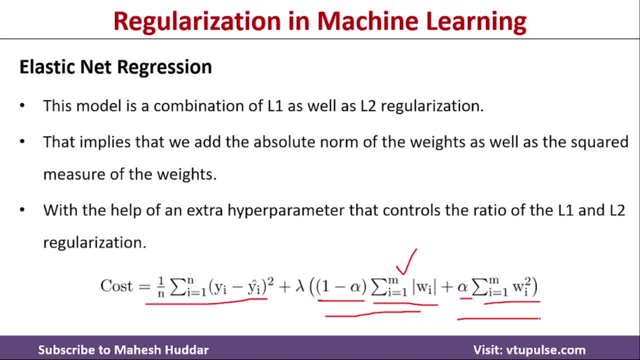 lasso regression. if alpha is equivalent to 1, we have something called as the ridge regression here. if the alpha value is anything in the range of 0 to 1, it is known as elastic rate regression over here. i hope the concept is clear. if you like the video, do like and share with your friends. press. 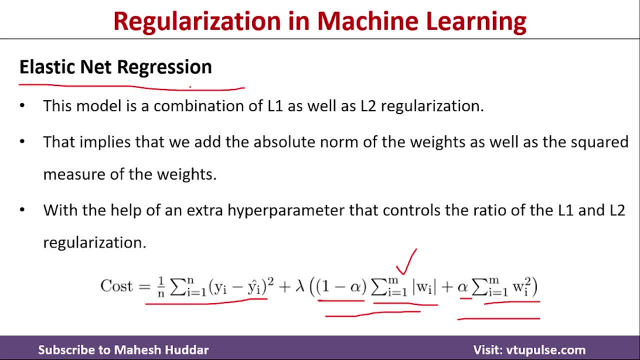 the subscribe button for more videos. press the bell icon for regular updates. thank you for watching.